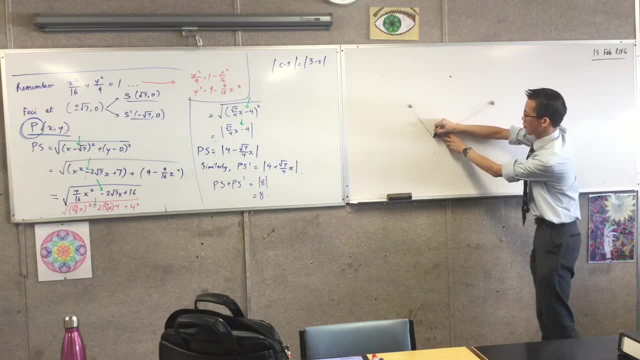 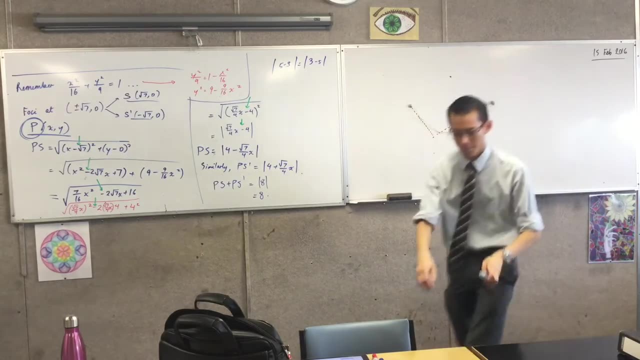 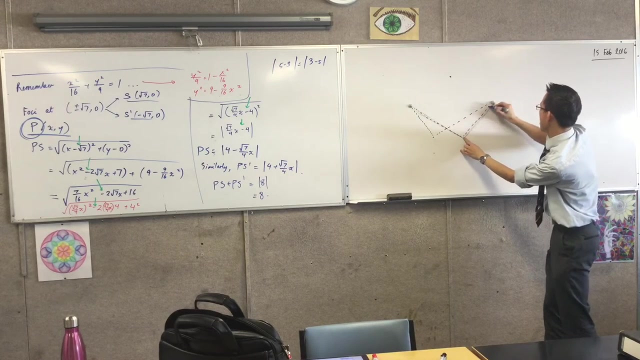 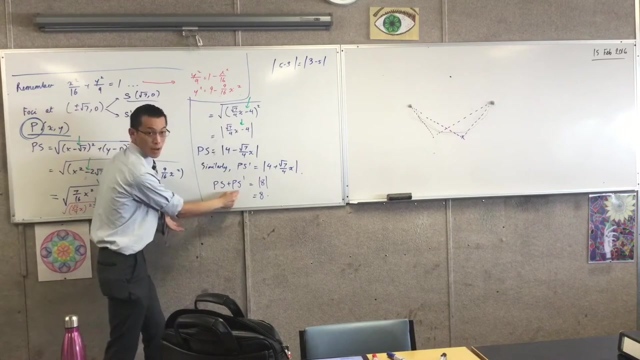 That point there, right? I'm going to even do some dotted lines here And that point right there, and let me get another cut This point over here. Do you agree, right, that those two points have the they exhibit this property, right? If I add them up, the sum of those two lengths is just. is just what the string is, right. I'm just moving it around, okay. 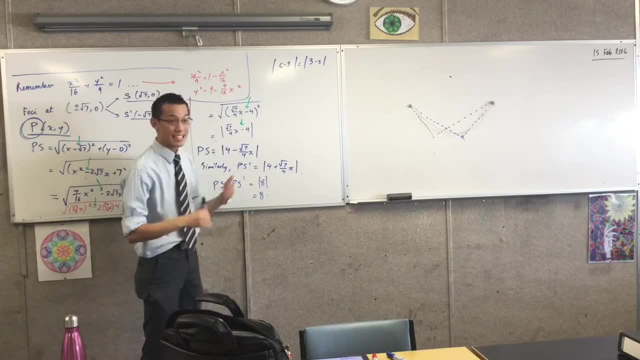 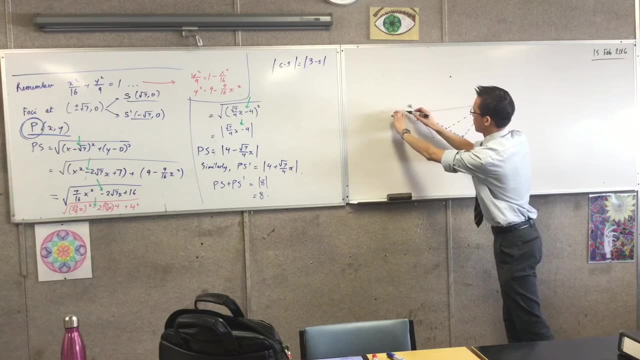 So I tried to practice, but I still find it quite hard. Let's see what happens if we trace out the locus of those points, right? So I'm going to start from over. I'll start from here. Let's see if this will work okay. 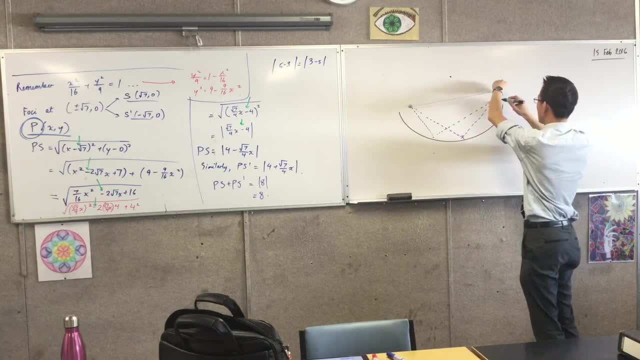 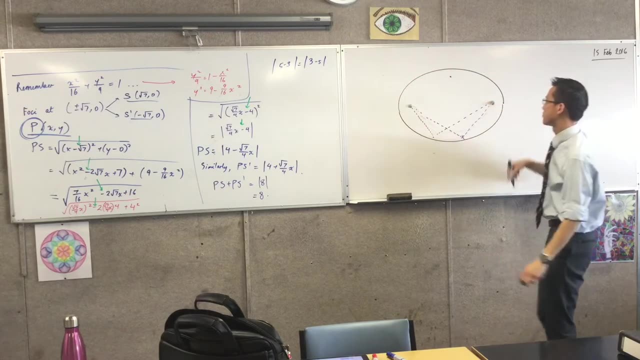 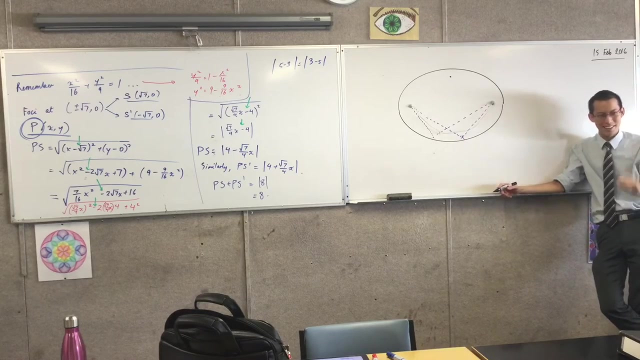 That's so cool. I got pretty close. You get the idea. That's good. Did you think about yourself? So? so conclusion: I'm going to bring string and Blu-Tack to an end-to-end. I've been having so much trouble drawing ellipses, why didn't I just now? what have we just established? okay? 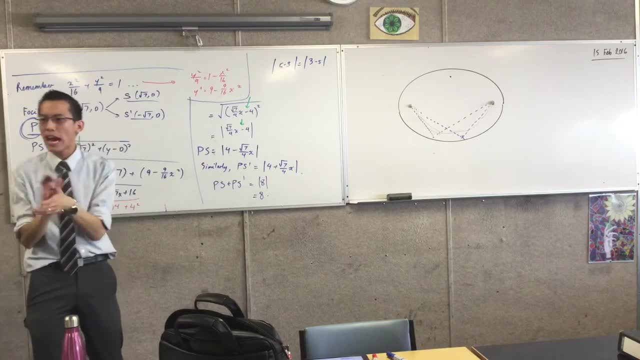 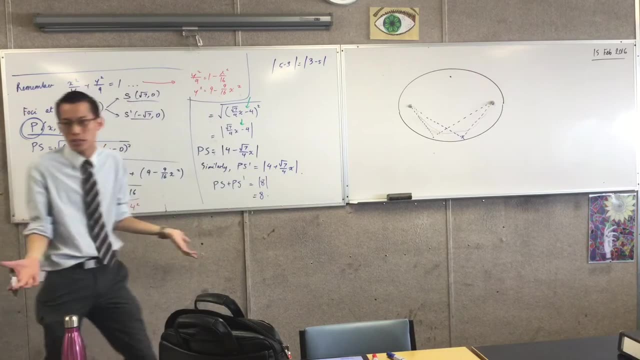 We have shown that we started with how do we start with the equation of the ellipse. We started with the parabola and then we said: let's muck around with the proportions, the eccentricity right. So in other words, we had not just P, S and D, but we also had P? D. 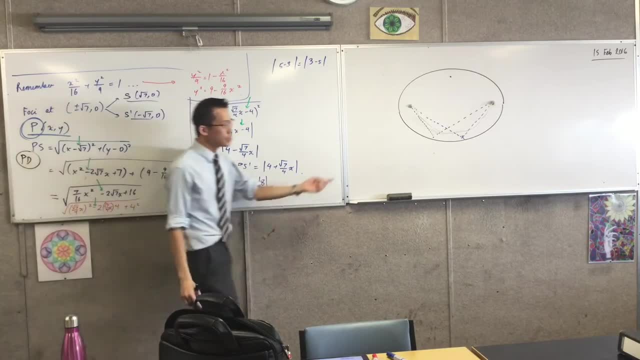 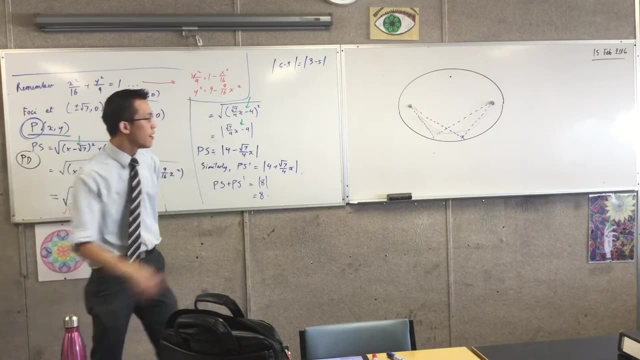 we crunched the algebra and out popped out the equation. This is a whole different way of doing things, right. And this, by the way, is what makes the Whispering Gallery work. Does that make sense? right? The reason why, if you're standing here, 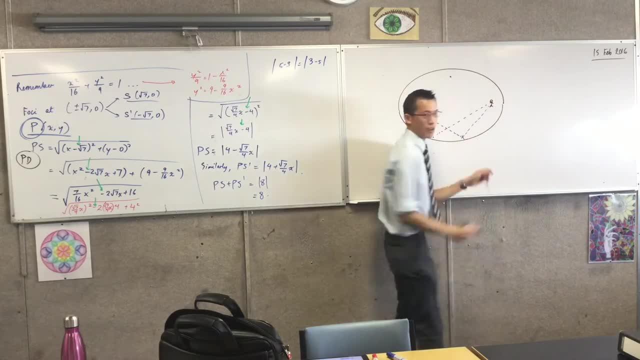 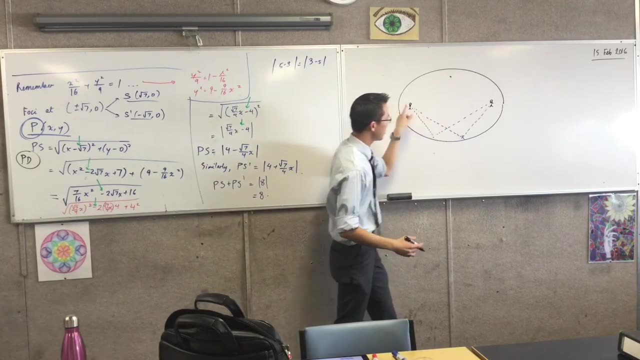 and you whisper to the person standing here, right? the reason that it works is because all of the sound waves that are coming from you are going to travel the exact same distance, no matter where they bounce on the walls or the archway of the Whispering Gallery, right? 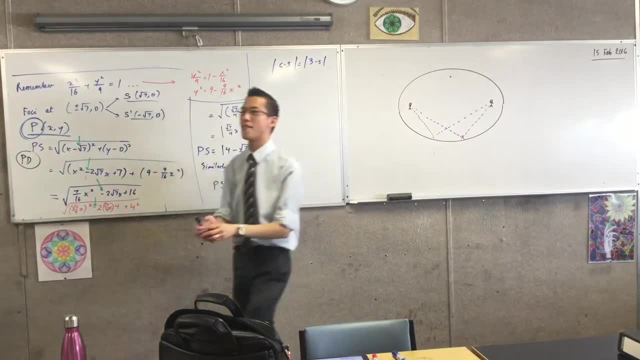 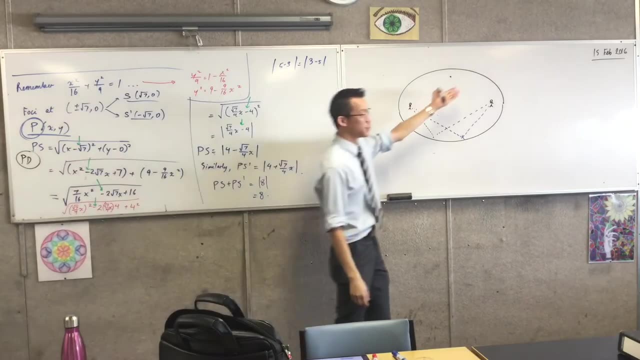 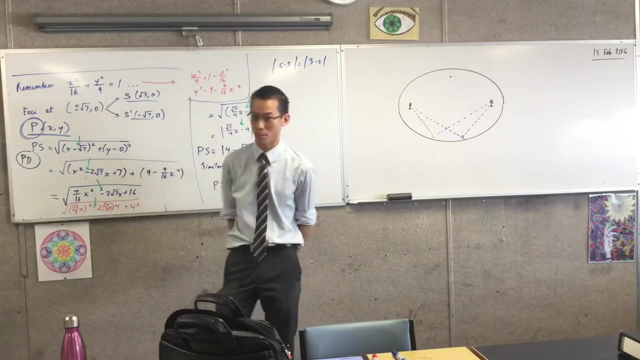 So, being that they travel the same distance, the sounds arrive at the same time, right At the same instance, because in that space, sound is going to travel at that rate, and so they arrive at you rather than scramble, which is what everyone in here will hear. right, They will hear exactly crystal clear, even if you whisper, okay. 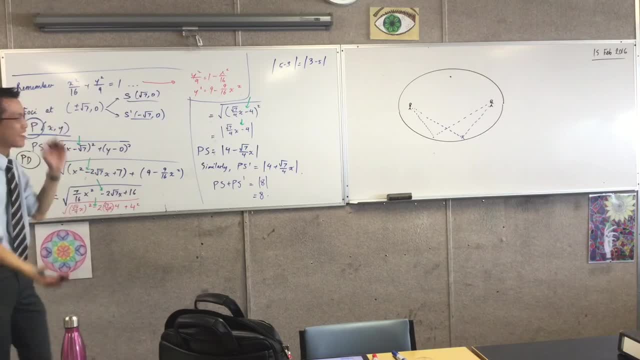 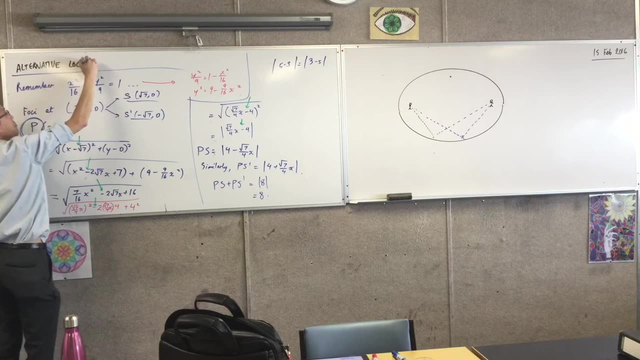 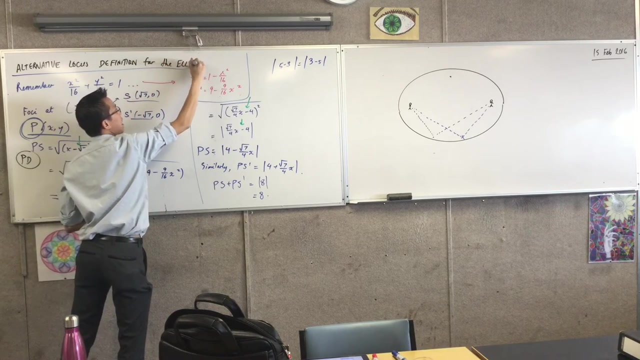 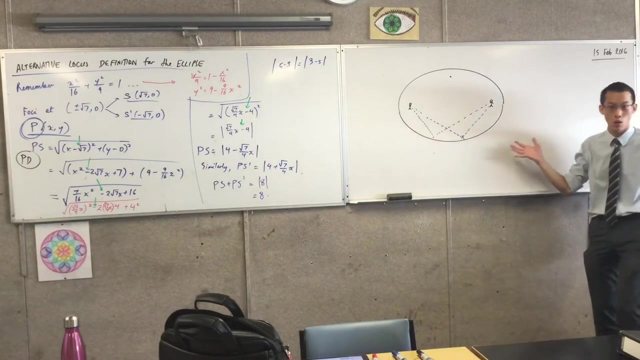 So, therefore, now we can make a heading. What have we just established? okay, What this is is an alternative locus definition for the ellipse. It is a whole other thing. It is a whole different way of arriving at the equation of an ellipse and at noticing one of its most critical properties. 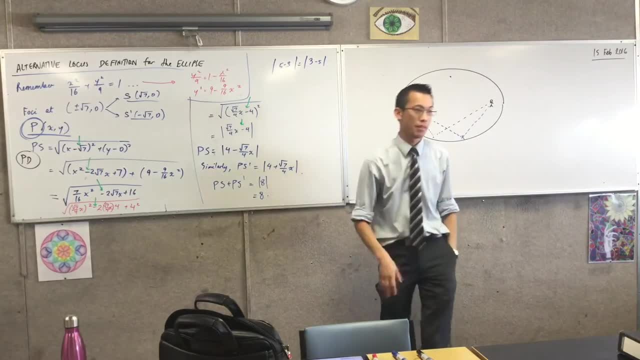 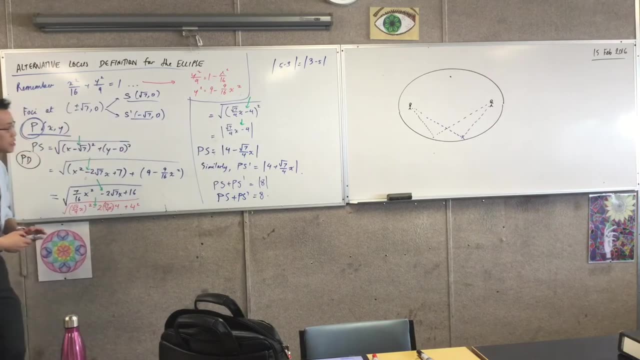 Now I want you to pause. We did all of this through like proper, actual numbers, right? I said that it would be substantially easier. You really actually do need to do this algebraically, because then you will see that this 8 is not a coincidence, right? 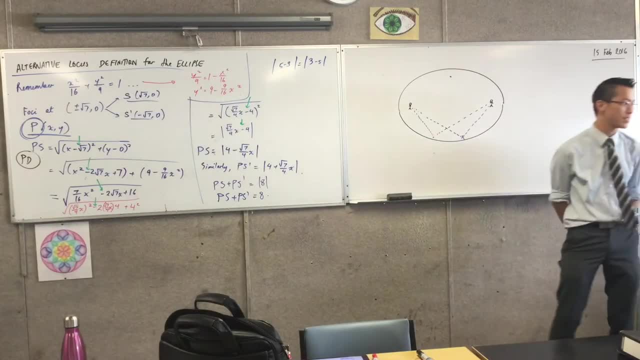 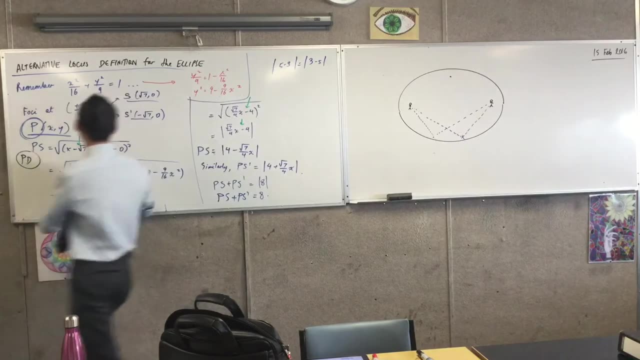 It's not just 8 randomly. Now if you look carefully you might be able to guess at what 8 is and what connection it has to the number that I've got here. Now if you're really really intuitive you'll see here's a right. This is 4 squared and this is 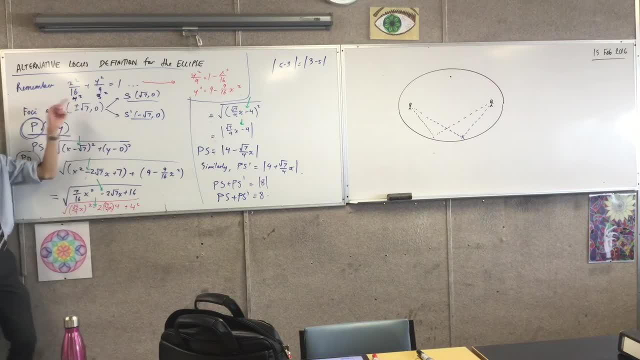 9,, which is 3 squared. Now why is it that the 4 squared comes into play? Why is it that 4 is what ends up coming out in my factorization? Because when you make the directrix and the profile like, the only thing that you talk about is a. 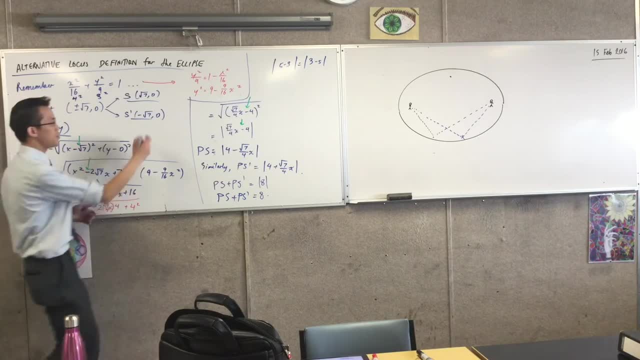 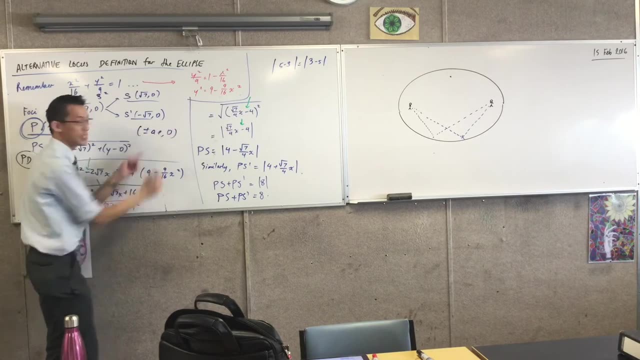 Very good. It's all about the major axis, right. You've got your. well, in this case we didn't deal with the directrix, but it's still the same thing. I've got plus or minus ae comma 0, right. 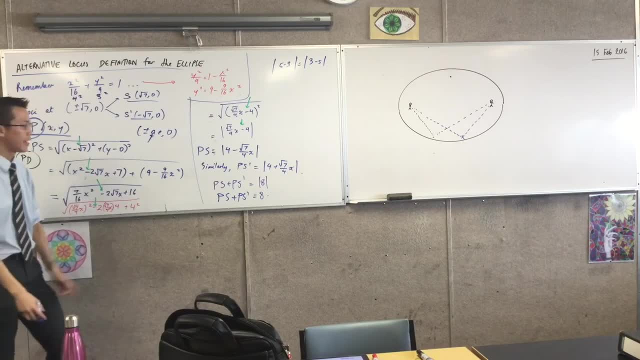 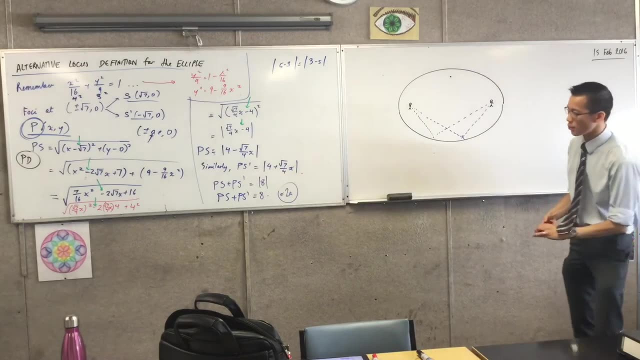 As you see, the major axis is where all the action is happening. okay, So this guy in fact here is not just 8 by coincidence, It is in fact 2a, and that is an important result to prove. Now I'm going to come around to you guys shortly. 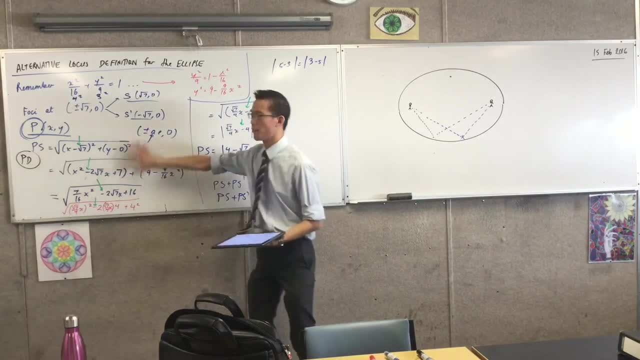 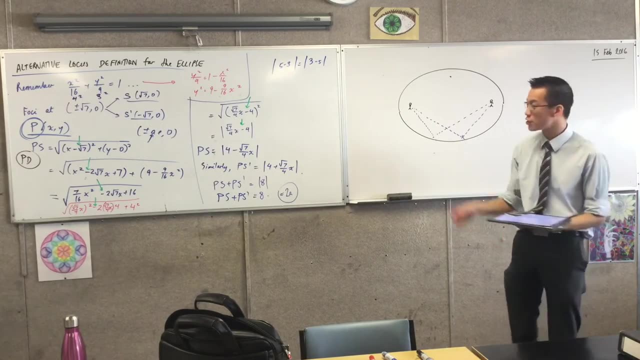 Because this is all numbers right. A lot of stuff is simplified out, but when it's algebra it doesn't simplify out. They're just terms and they don't coalesce. They're not like terms. You have to do a lot of. 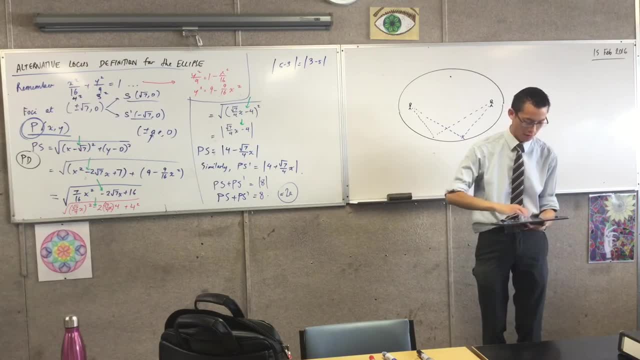 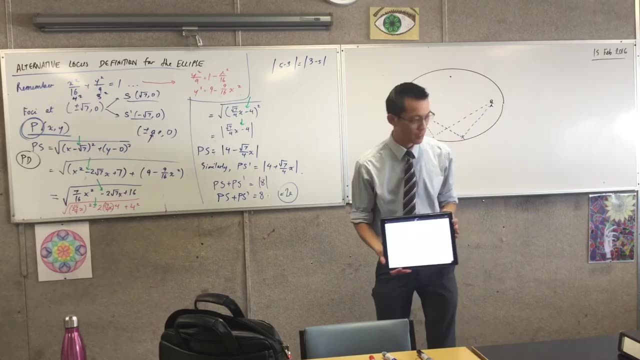 massaging of the terms and your proof ends up about about that long. Now that doesn't look too long, but a lot of the steps- and I'll come around and show you this in a second. a lot of the steps are like: why would you do that? Like: how on earth did you know to do that? 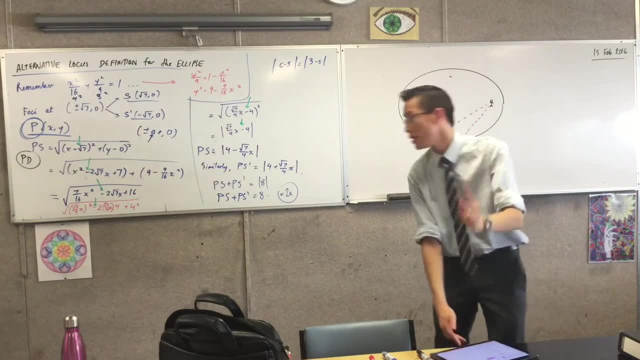 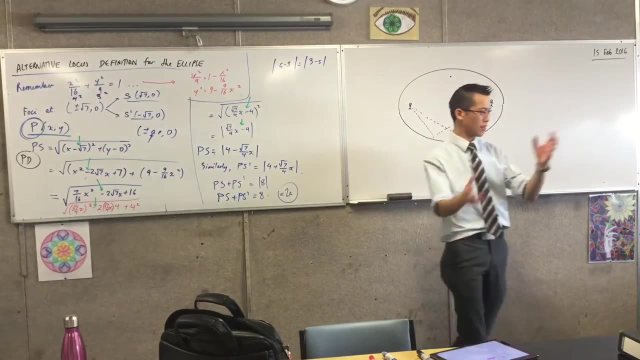 Like what made you do that particular algebraic simplification? And the answer is: when mathematicians go through this and they're like huh, pattern, There must be a pattern in here. Then, when you go to the abstract, the algebra, you're like: okay, I'm searching for something, I'm not doing something like this, I'm just going to do something like this. I'm just going to do something like this, I'm not doing something like this, I'm just going to do something like this. I'm just going to do something like this. 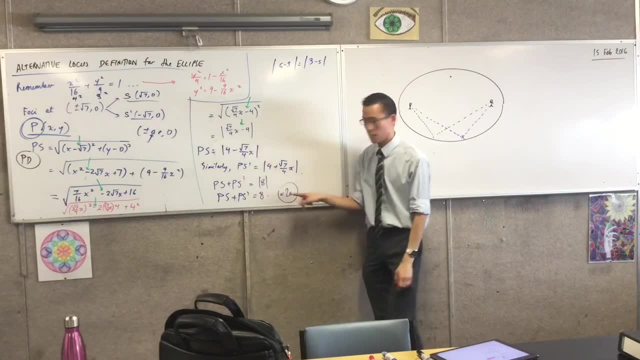 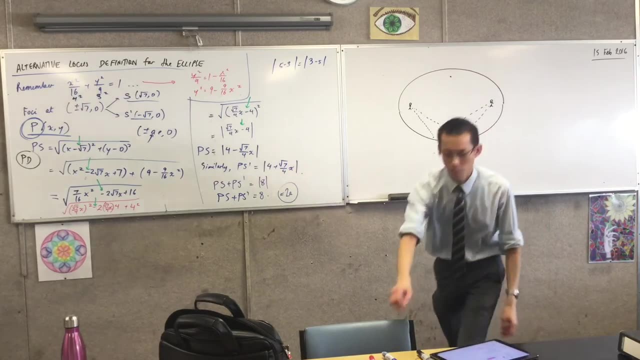 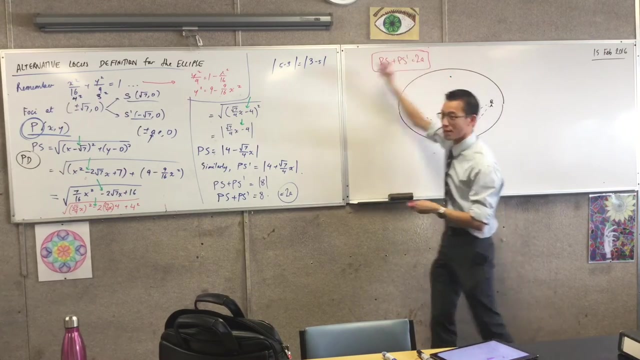 simplification, like at random. I'm after something specific so that guides the presence, just like a true identity when you solve you, okay, so I'll come around and show that to you. but this property here, let's put a box around it. PS- okay, it is oft forgotten because people focus on the other locus definition for. 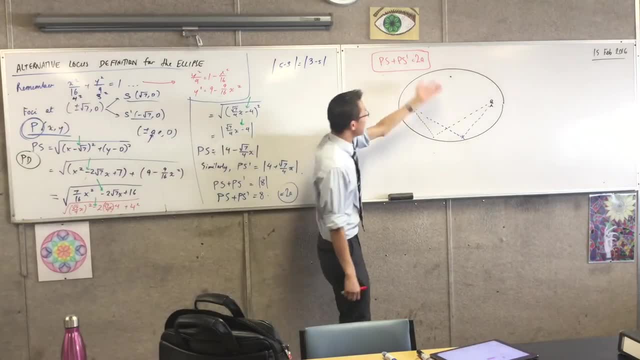 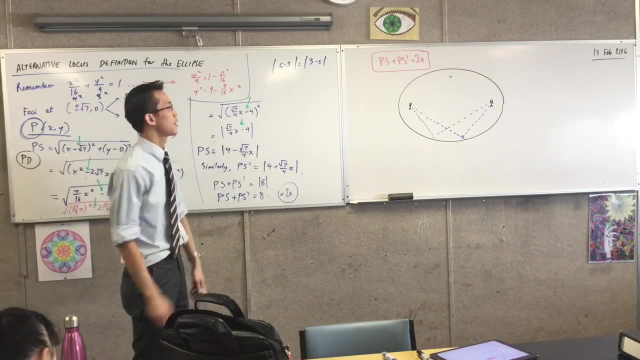 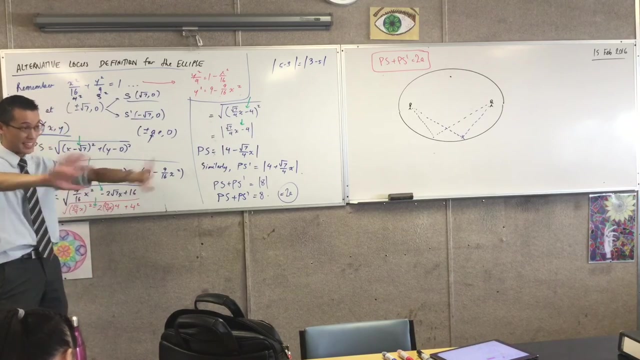 the ellipse, the main one. but this is- and I hope you can see it is- beautifully simple, right, and so you therefore can get lots of geometric insights out of it because of how easy it is right. some of the questions in 4.1 all right now, like 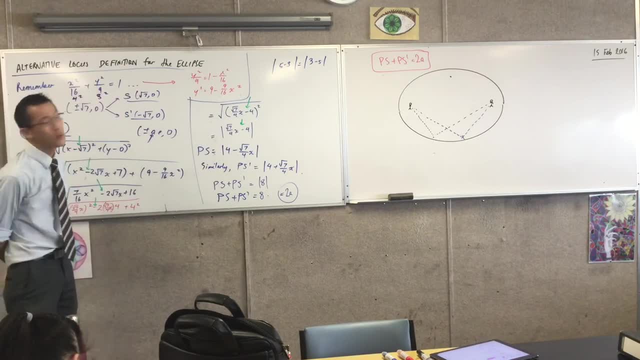 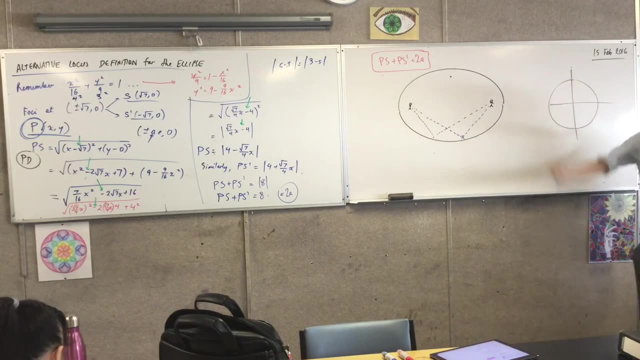 I said that's all of the basic stuff for ellipse. we will revisit the ellipse and we have a look at. we got, we know and you can probably guess at this right. if I give you the unit circle right, I can stay any point on the circumference in. 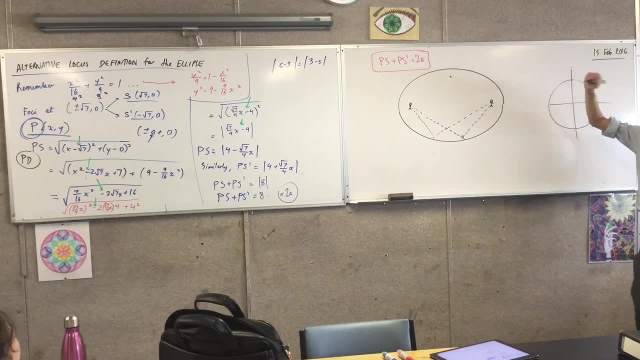 Cartesian terms, so being that this is the unit circle, what's the equation of the unit circle? good, so in Cartesian terms, I would state this as X comma, plus or minus, the square root of 1 minus Y squared, and the plus or minus depends on whether I'm on the 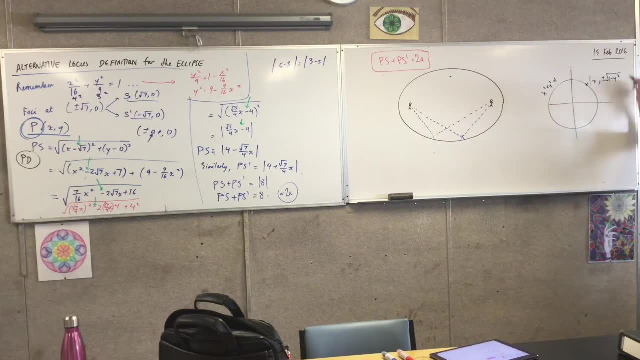 top semicircle or the bottom right, so that's in Cartesian terms. but of course we know the only way you can do it. how else would you do it? yeah, we use cos and sine. so that is the way we would parametrize, we could express it. we can do the same thing for the ellipse, in fact, because 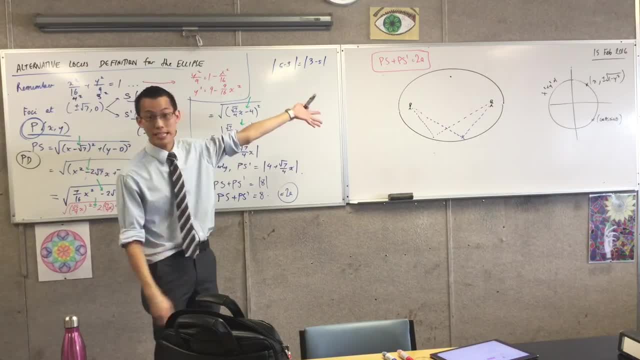 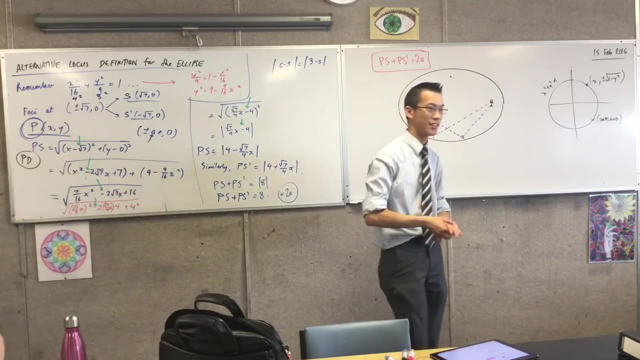 the ellipse in the circle, so closely related they're almost identical. okay, we will come back to that a bit later on. we're a bit further into phonics, but for now, hooray, ellipse is done.